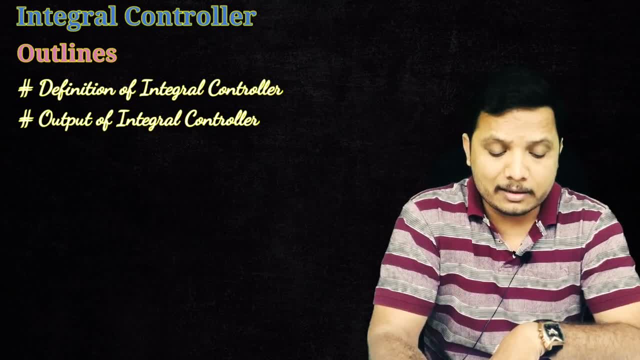 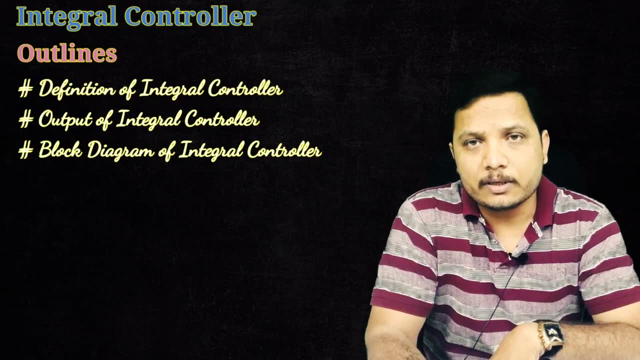 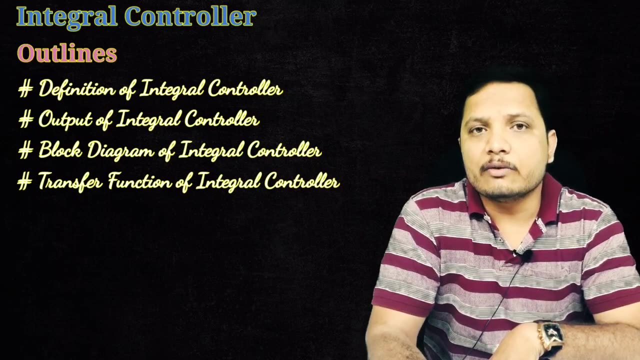 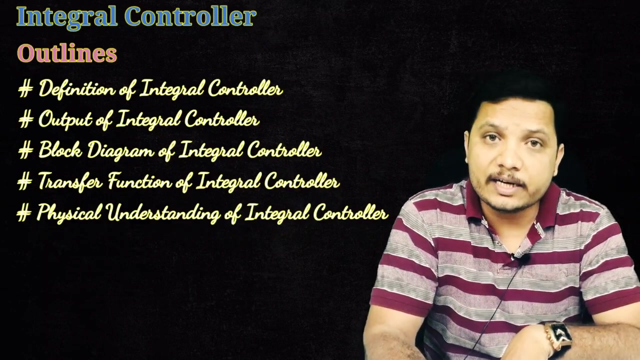 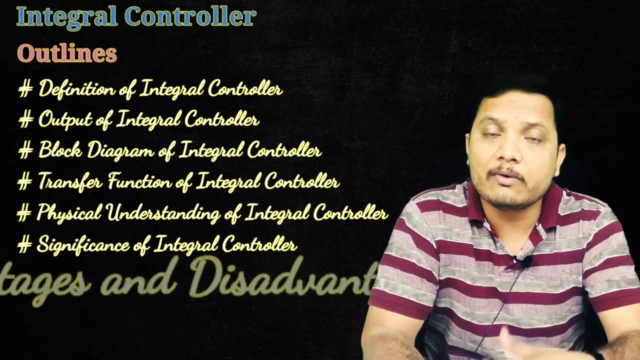 is there with integral controller. Then we will see block diagram of integral controller with second order system. Then I'll explain you transfer function of integral controller with second order system. After that we will see physical understanding of integral controller. Then we will see significance of integral controller and at last we will see how advantages 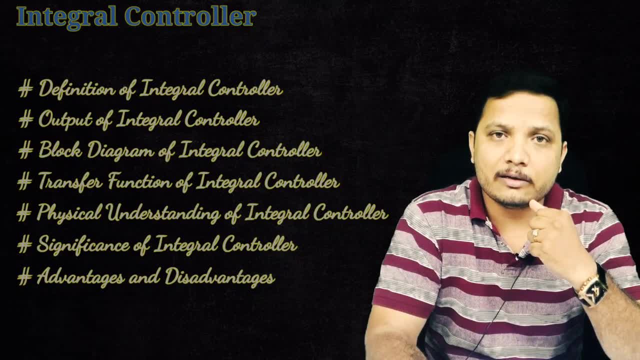 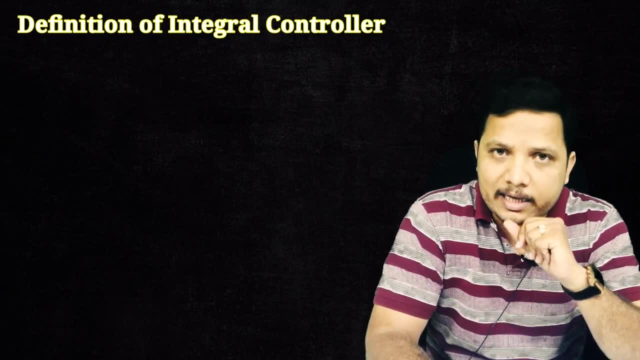 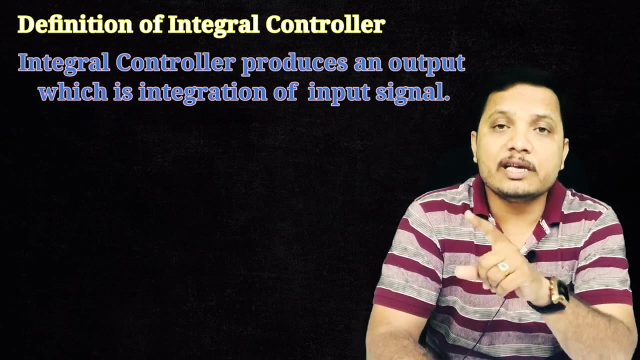 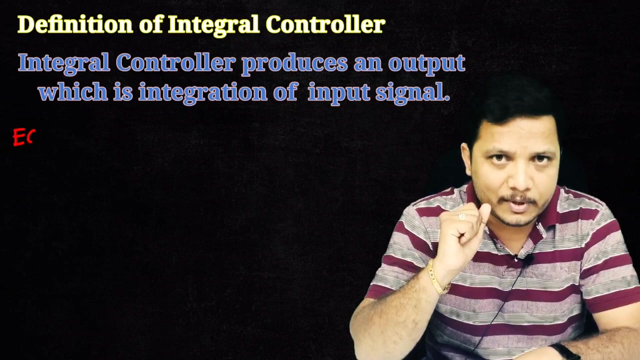 and disadvantages are there with integral controller. So let us begin this session with first agenda, that is, a definition of integral controller. Now you see, integral controller means output of integral controller will be integration of input which is given to the controller. So let us say we have integral controller over here. you can see, and if I give input signal that 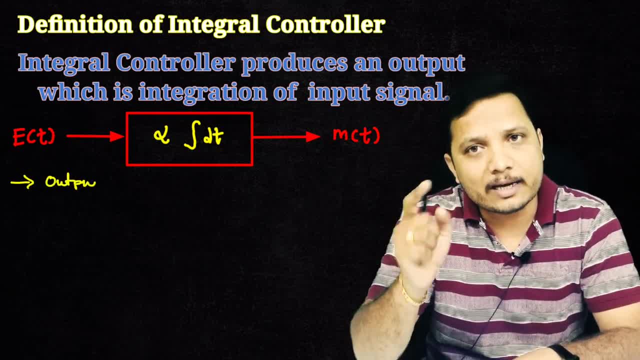 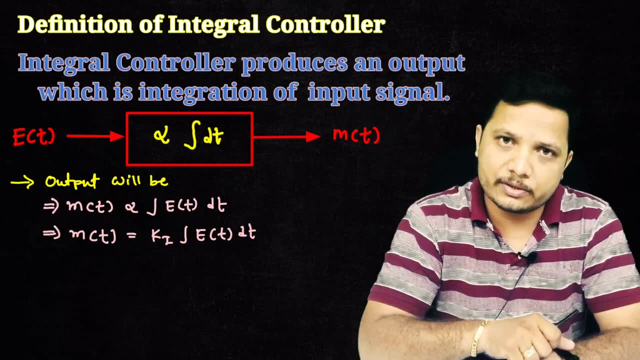 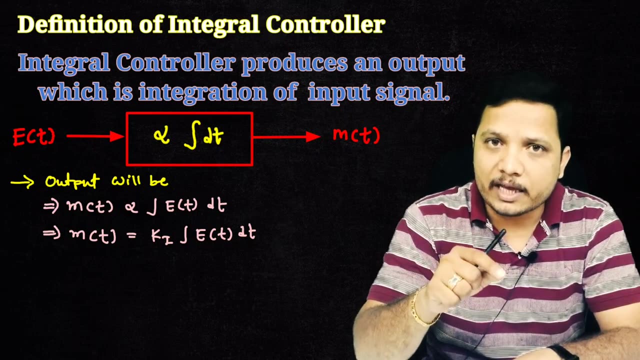 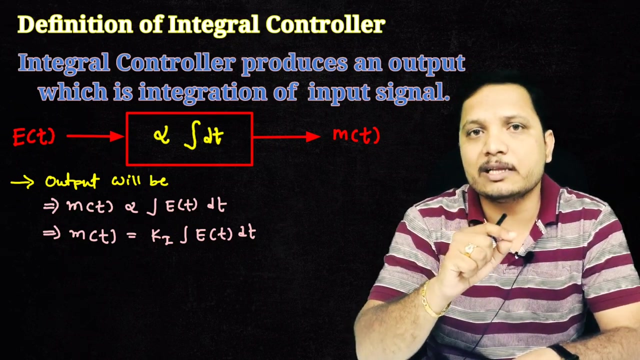 is e of t, then output of that integral controller will be integration of e of t into some proportionality constant. So here, if I say my output is m of t, then m of t is directly proportional to integration of input that is e of t and this proportionality. 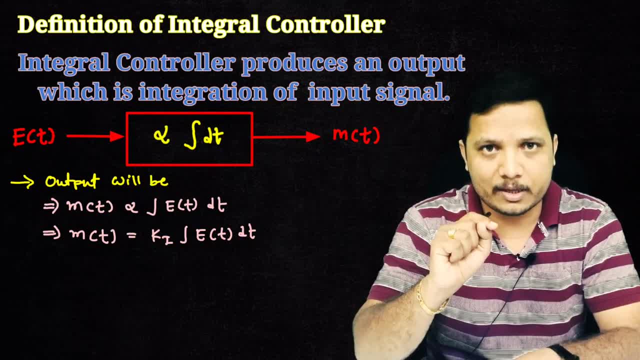 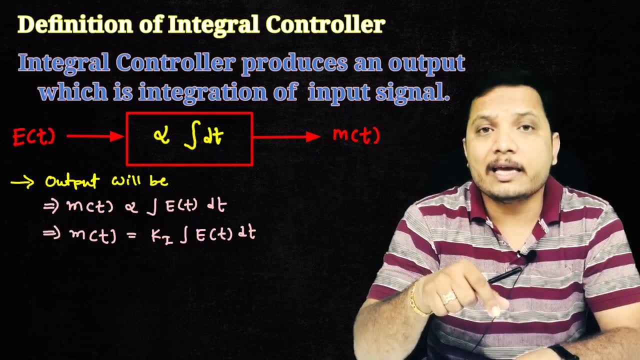 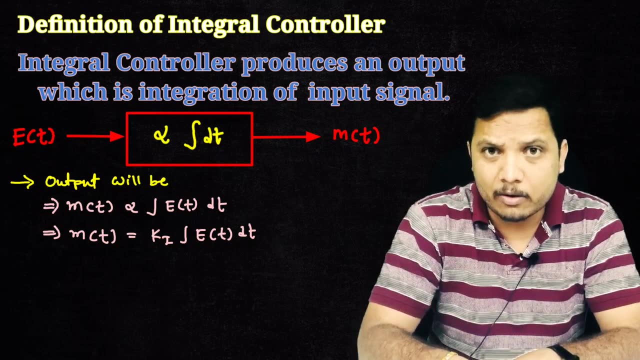 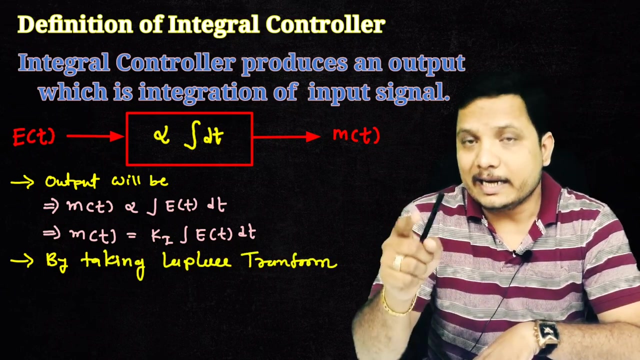 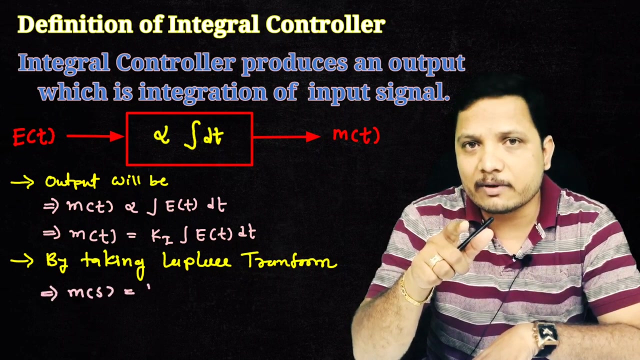 controller for integral controller is k i. So my output of integral controller is m of t is equals to k i into integration of E of t. Now here, if you take Laplace transformation of this, in that case that integration that is resulting into E of t integration is equals to E of s divided by s. 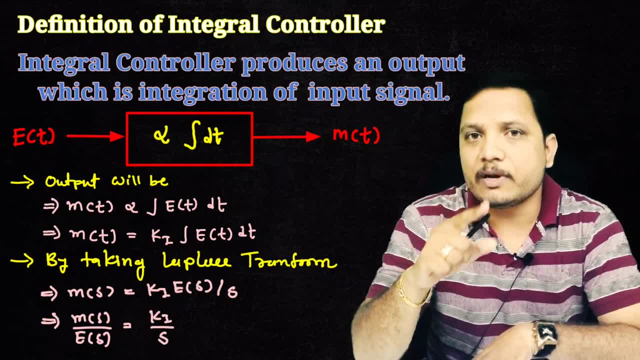 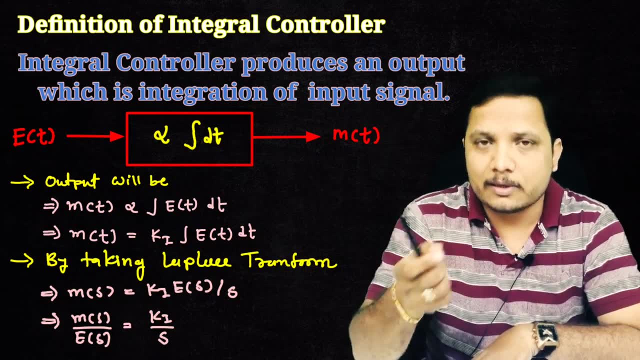 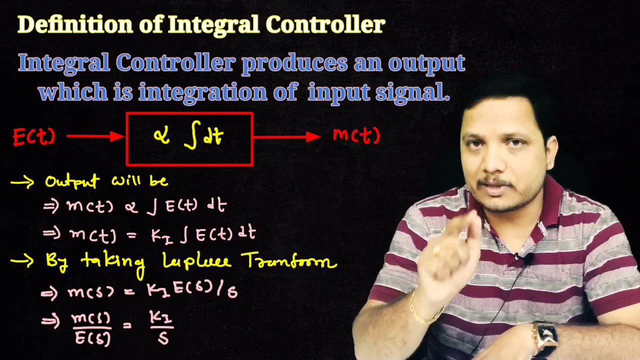 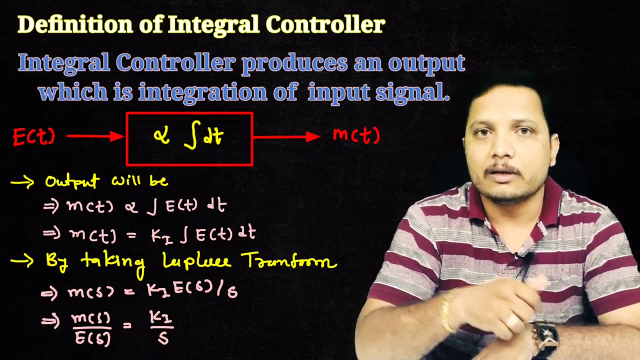 So the transfer function of integral controller, that is output, which is m of s divided by input, that is E of s, that is ki divided by s. So that is how output is happening, as per the basic definition of integral controller. Now let us try to understand this. 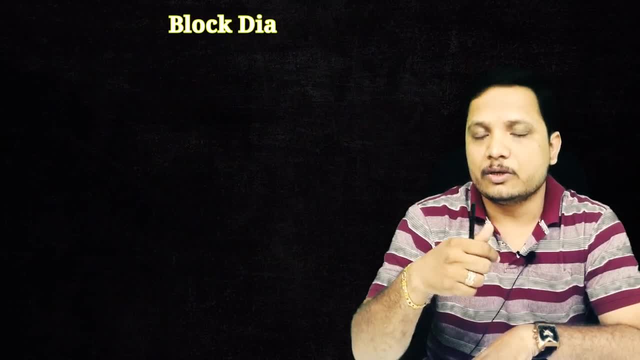 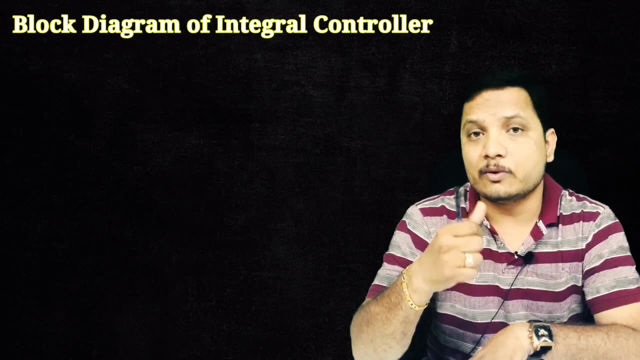 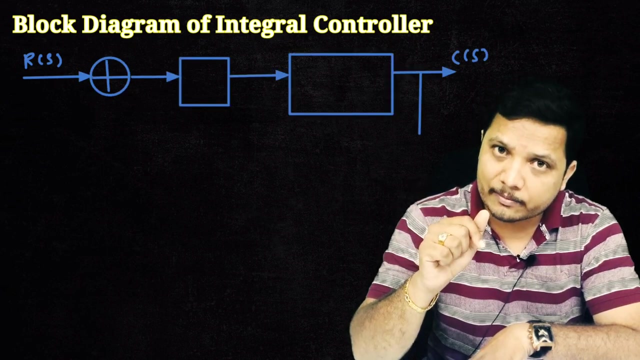 by second order system. So here I will be considering a block diagram of second order system with integral controller. So first of all you just see the basic block diagram which is there with control system with negative feedback. Now in that that controller, that will be integral controller over here. 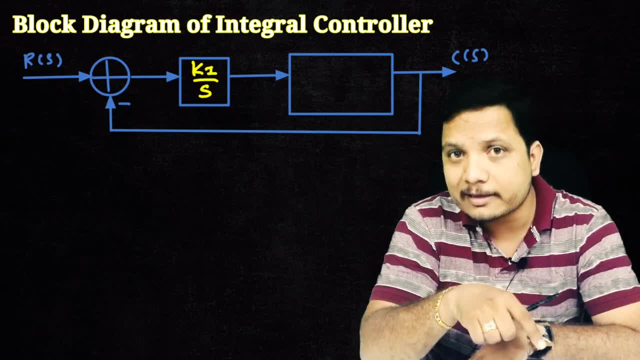 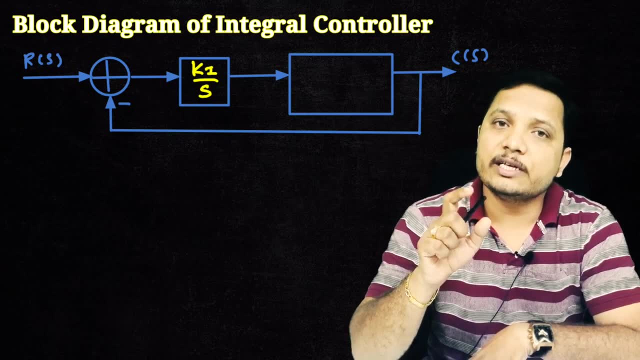 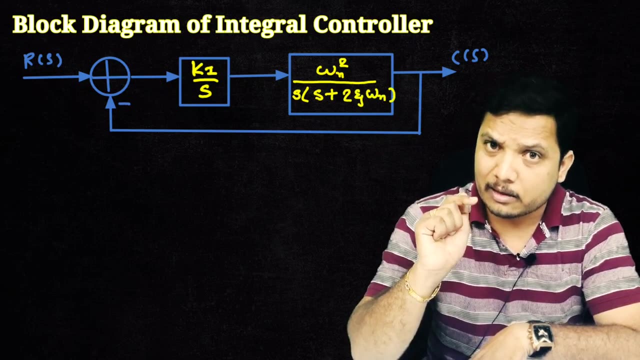 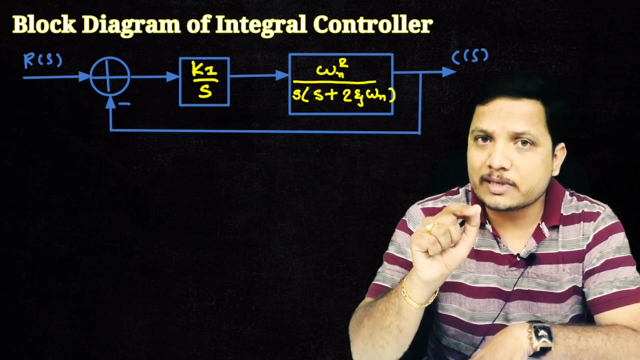 So integral controller is having block diagram that we have calculated recently. that is ki divided by s and second order system transfer function is omega n square divided by s into s plus 2 zeta omega n. right now, if you calculate this transfer function by simplifying it, then you see ki by s and omega n square divided by s, s plus 2 zeta. 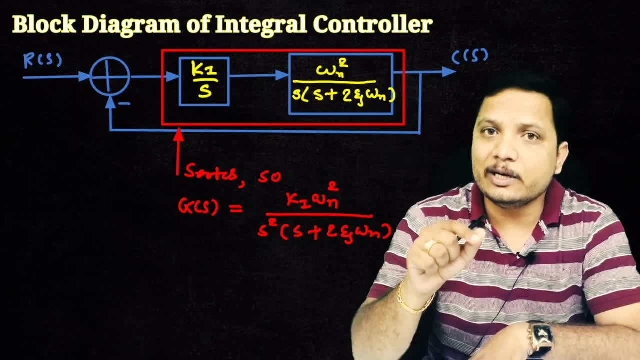 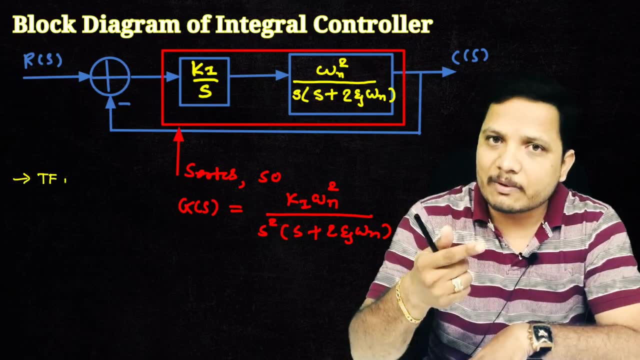 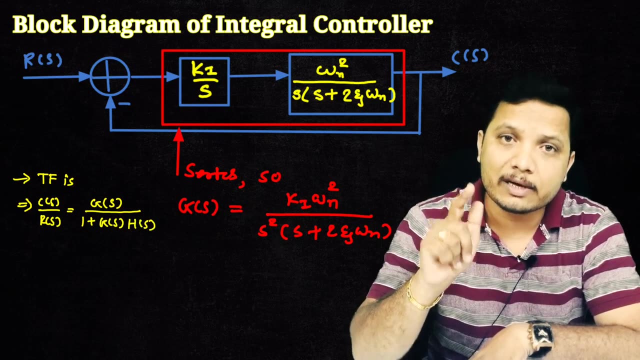 omega n that is there in series. so that is resulting into multiplication of these two term and this is negative feedback system. so transfer function of negative feedback system is gs divided by 1 plus gs, hs. here hs is equals to 1. why the reason is this is unity, negative feedback. 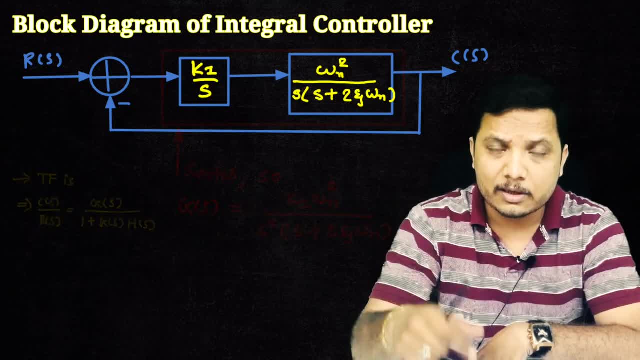 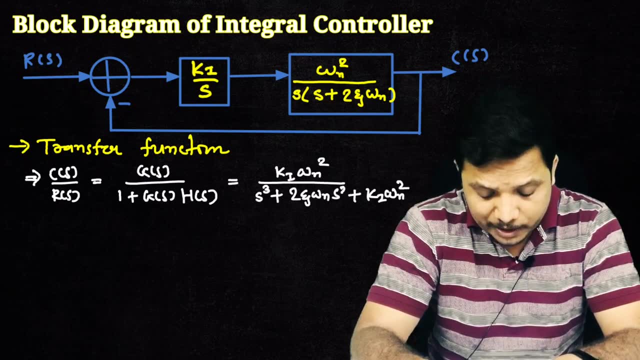 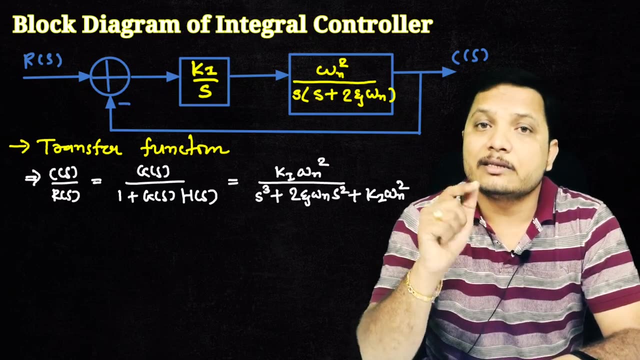 and if you place these values, your transfer function, that will be ki omega n square divided by s cube plus s square 2 zeta, omega n plus ki omega n square. and if you compare that with standard second order system, that is omega n square divided by: 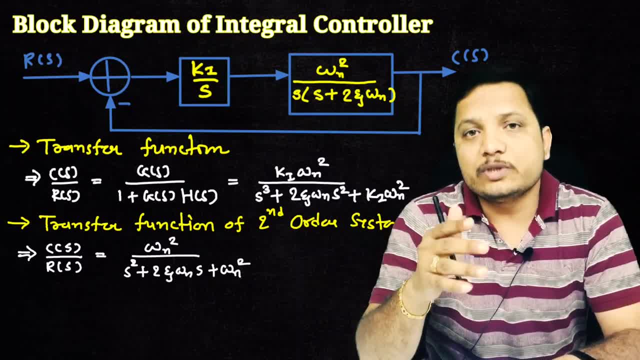 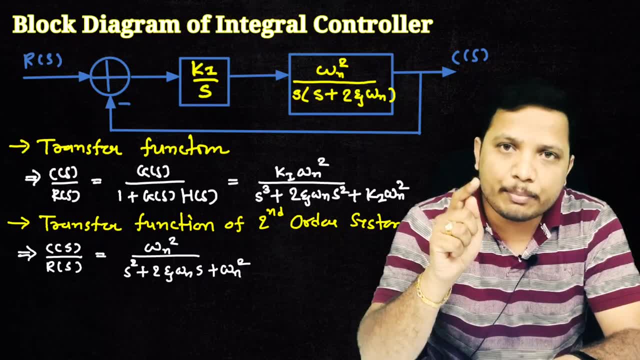 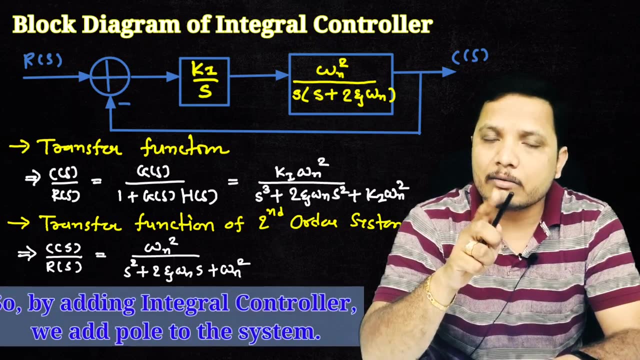 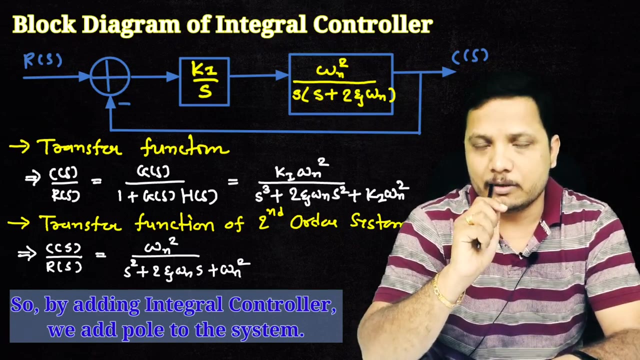 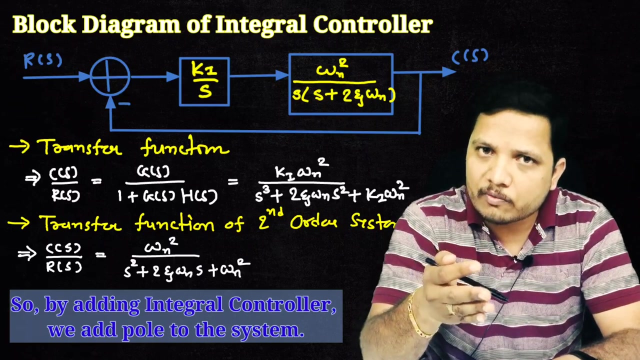 s square plus 2 zeta, omega n s plus omega n square. then here you just see, we have added one pole to the system by adding integral controller. so if you add integral controller, what we do, we add additional pole with the system. so, without integral controller. order of the system was 2 with integral controller. 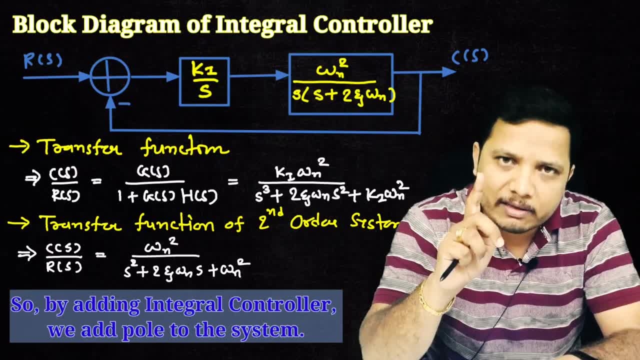 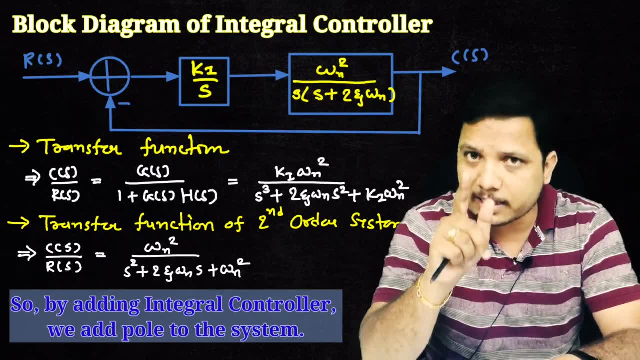 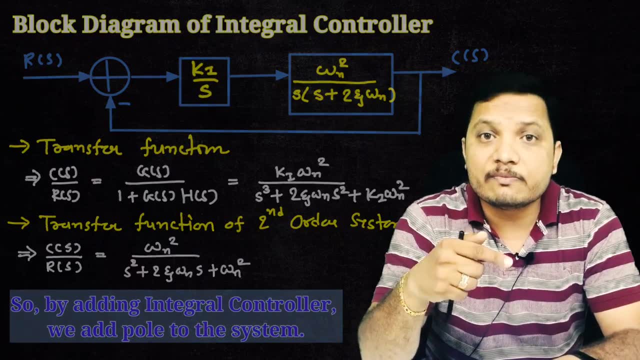 now order of the system is 3. means additionally, we are adding one pole to the system. means stability of the system will decrease because of integral controller. this is one thing that one should keep in their mind. now let us try to understand integral controller first, with its physical understanding. 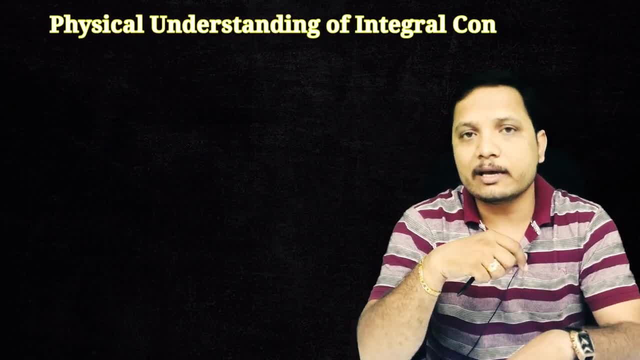 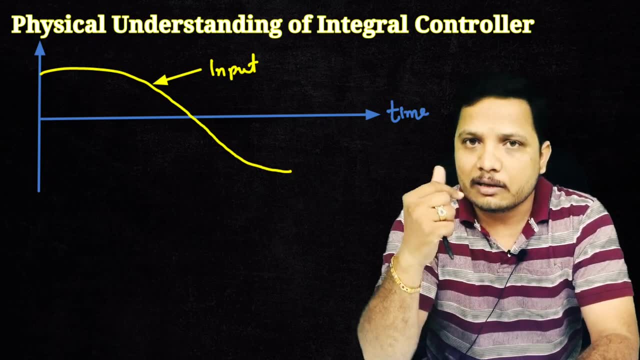 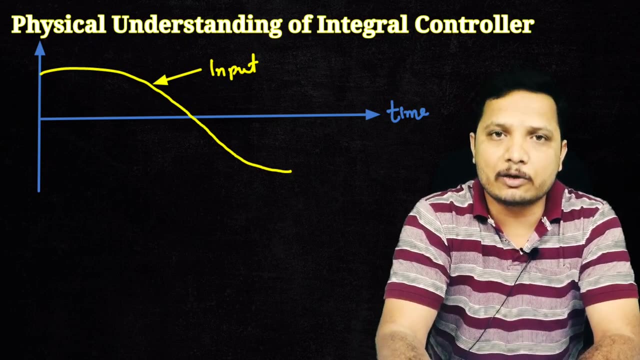 so it will give you bit more clear idea. so here we have integral controller with which we give input. let us say we have input with signal. that you can see it in graph here. i have shown the graph now how output will appear in integral controller. so see when we talk. 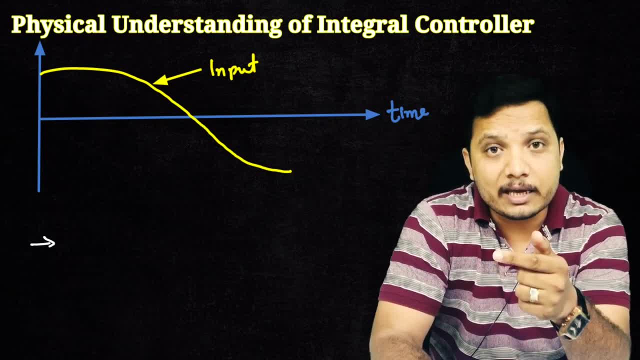 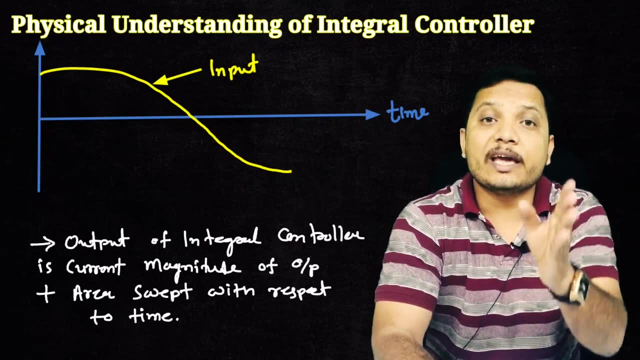 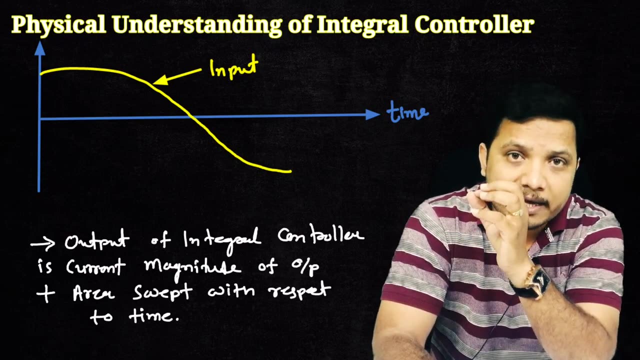 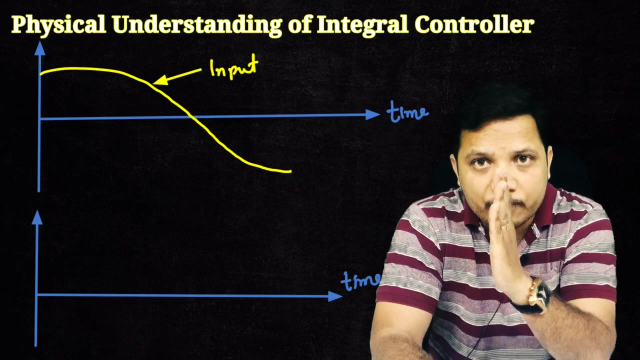 about integral controller, output will be current magnitude plus algebraic sum of area covered with respect to time. So initially, if I say my area is 0, so initially my output is 0.. Now, as I move further with respect to time, area should get added with. 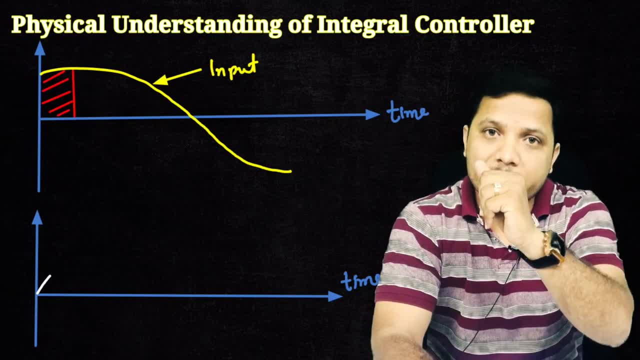 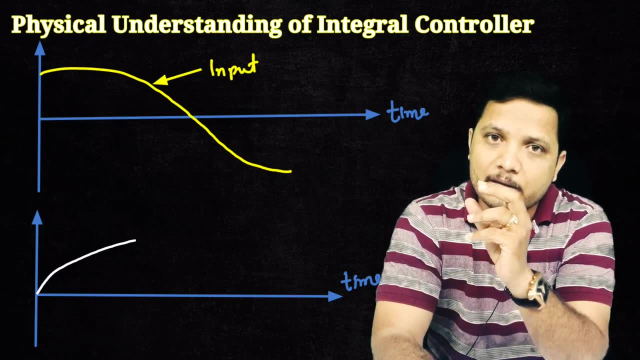 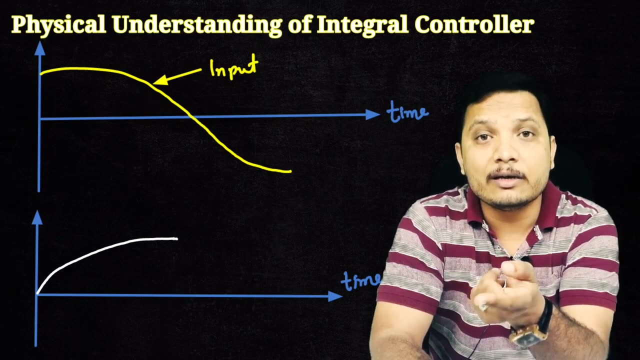 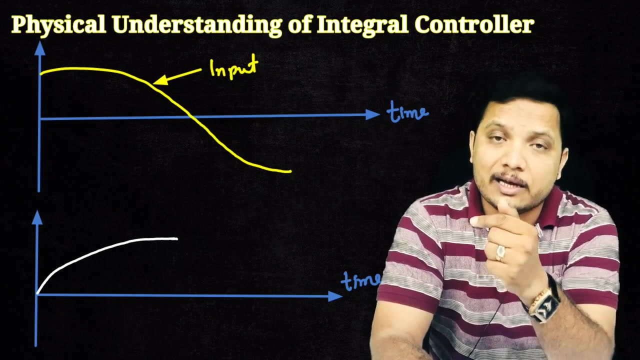 output. See above area is positive, below area is negative. So as you move with respect to time, if area is positive, output will increase. If area is larger with positive magnitude, output will increase faster. So that is how output will change and here you can see. at this point 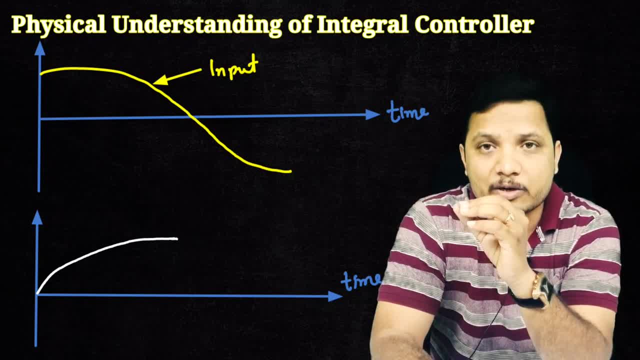 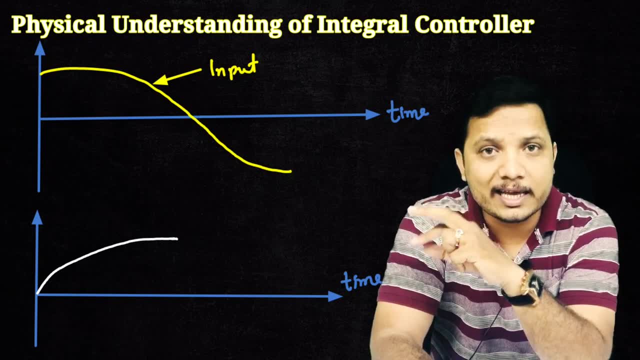 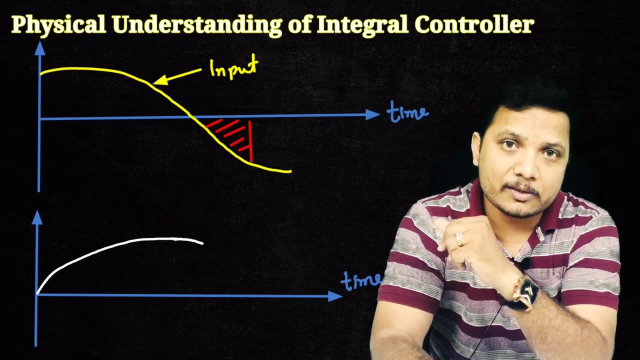 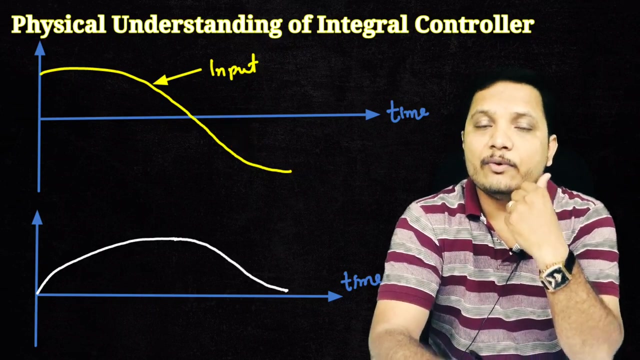 area is 0 with respect to time t, then output will not increase at that point. But after that point, if you see area is getting negative, means after that point output will start to decrease. So this is how output is coming in integral controller. So here there are few. 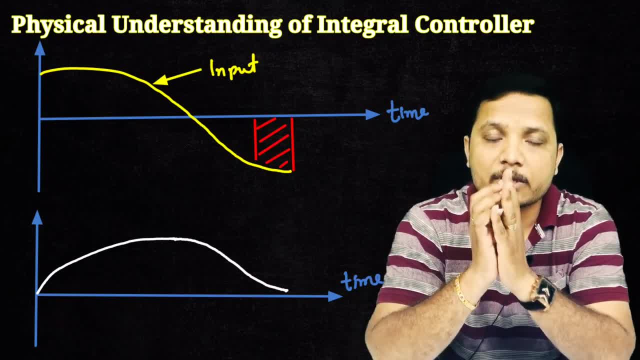 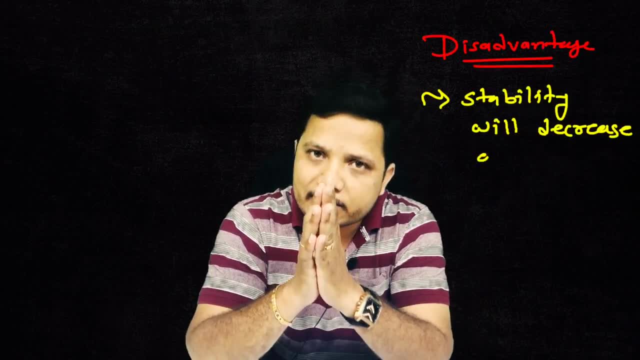 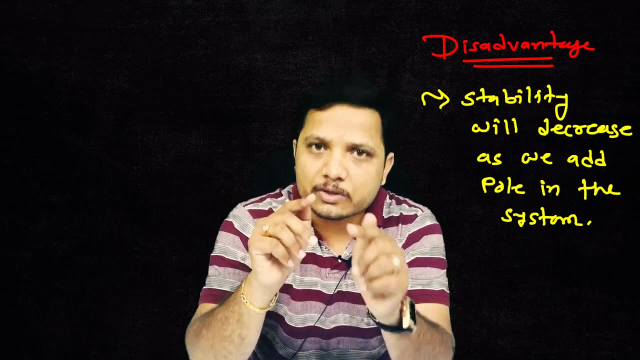 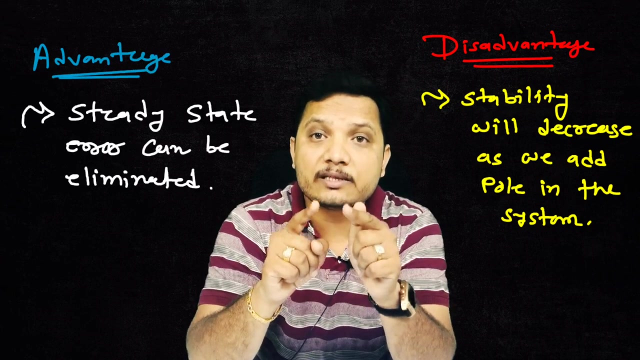 advantages and disadvantages that we should understand. See, in integral controller we add advantage and disadvantage. So in integral controller we add advantage and disadvantage to the system. and as we add additional pole to the system, system stability will decrease. But because of integral controller we can eliminate steady state error or one can say offset of the system in steady 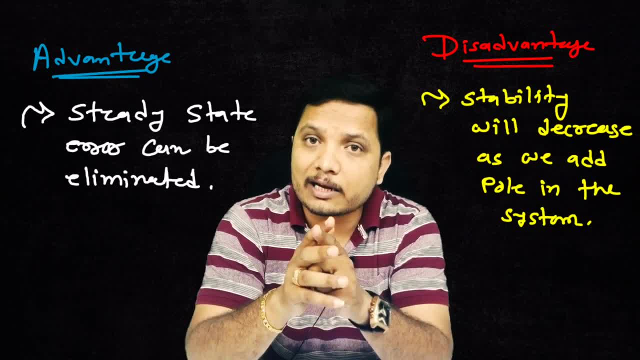 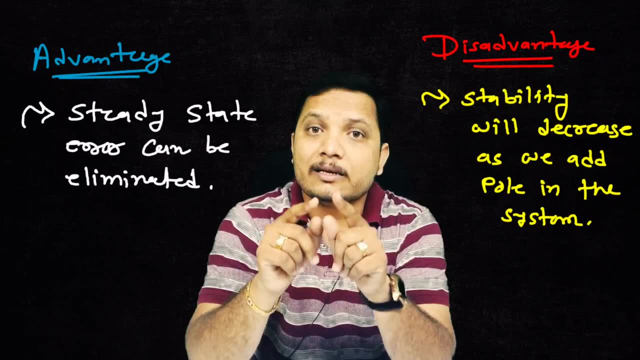 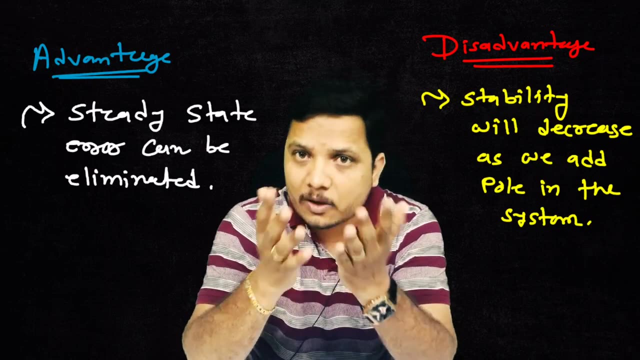 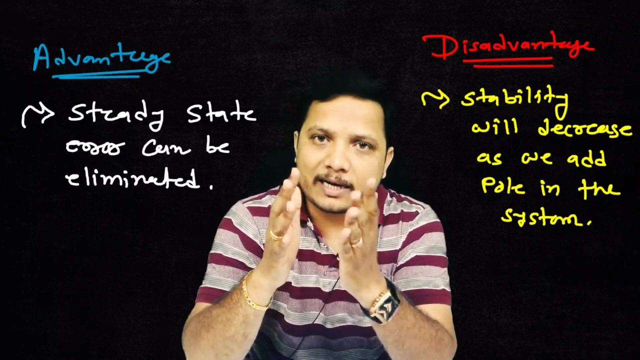 state output. So integral controller eliminates offset or one can say steady state error, but it also adds bit instability to the system as order of the system increases. So this is all about integral controller. I hope you have understood this. Thank you so much for watching this video. Just write down your comments. I will be happy to help you by writing answers. Thank you.